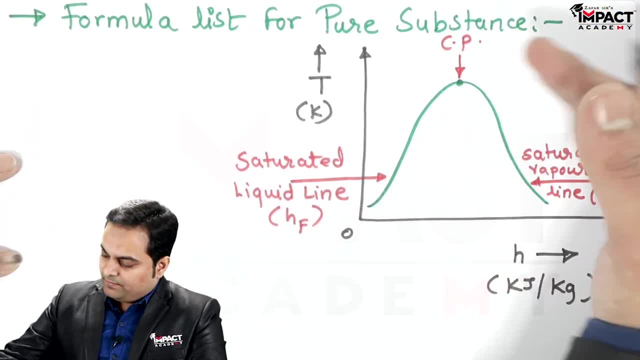 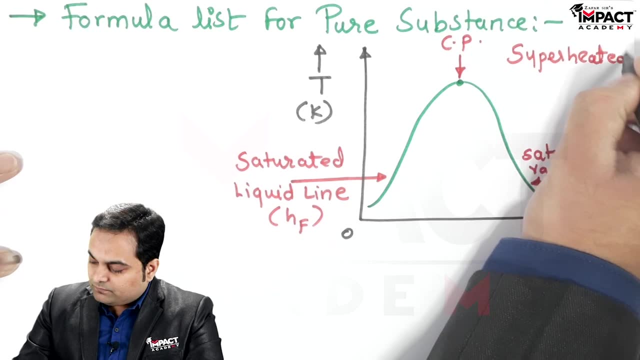 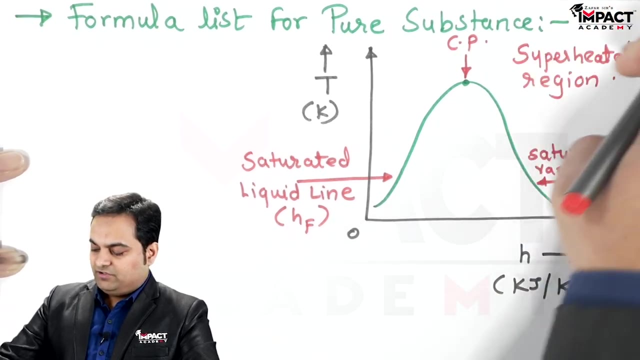 Next, whatever the region is there beyond the saturated vapor region, that is called as the superheated region. So this is the superheated region and whatever the enthalpy values we are going to get in this region would be called as the superheated value. 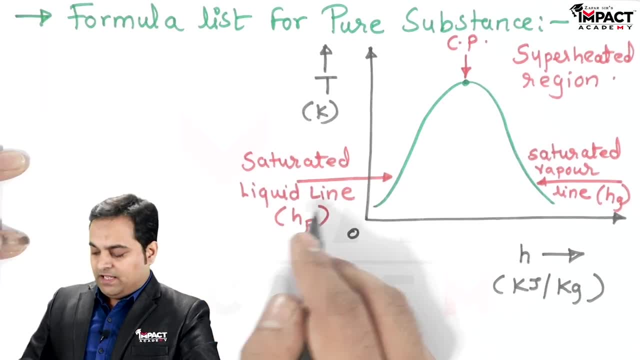 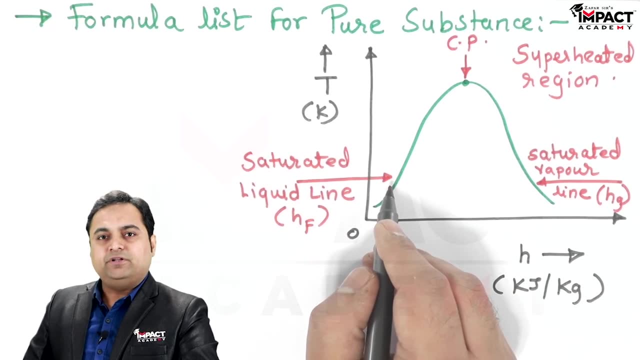 And what is the meaning of superheated? I explain it in this way, in the simple form: Like if we have water which is boiling at atmospheric pressure, Then we know when water would be heated. the temperature goes up to 100 degree Celsius. 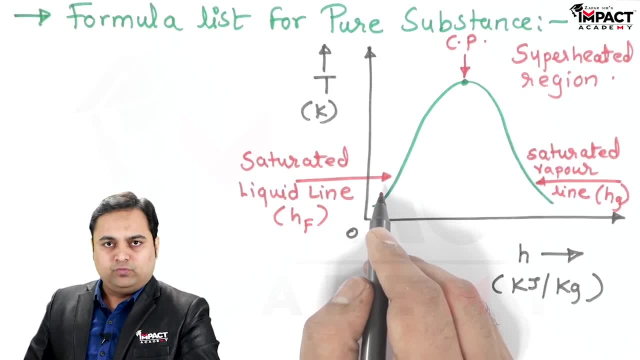 In that case, when it is 100 degree Celsius, water is entirely liquid, Then the enthalpy value would be called as hf, because it is saturated liquid line, Because water is now not converted into steam, That is, the conversion has not started yet. 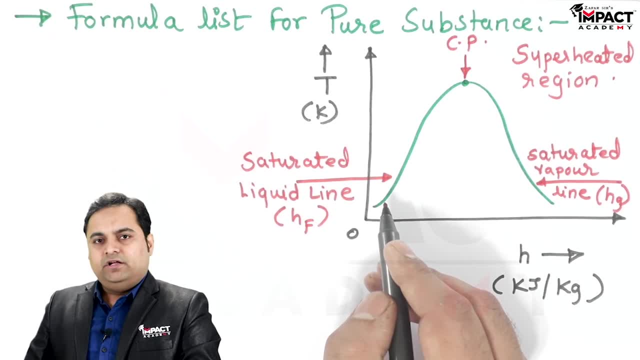 It is only boiling up to 100 degree Celsius. Then, the moment the temperature is 100, the phase change will take place, That is, the temperature won't be increasing from 100 to 101. At first, what will happen is water will be converted into steam at the same temperature. 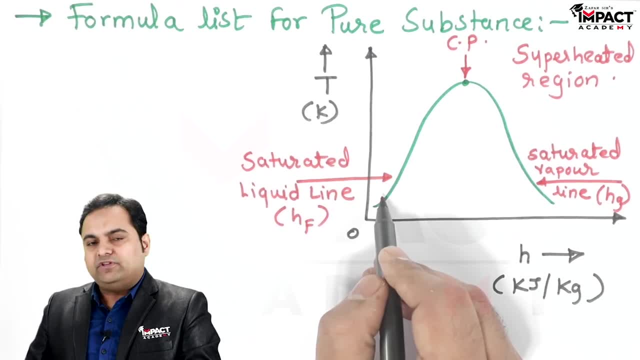 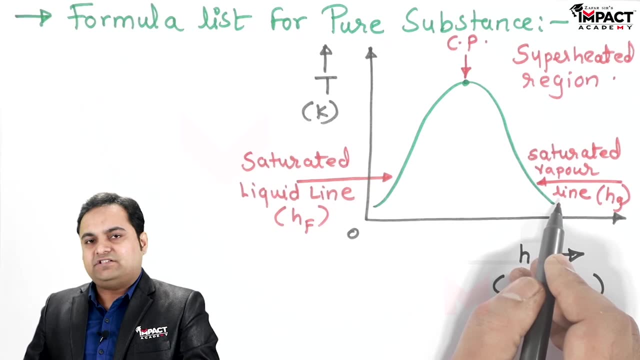 So saturated liquid line shows the enthalpy of that water which is boiling at 100 degree Celsius, And hg value shows the enthalpy of that dry steam, The water which has been converted into steam completely but the temperature is at 100 degree Celsius. 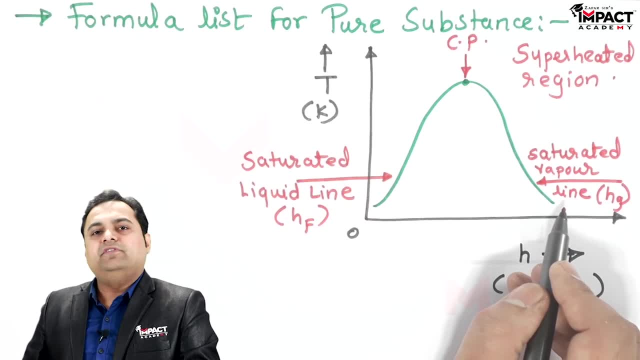 So that is the hg value And the moment we reach 100 degree Celsius, converted into steam completely, And when we try to increase the temperature above 100. That is, we can say 120 degree Celsius, 150 degree Celsius, Then that steam is called as the superheated steam. 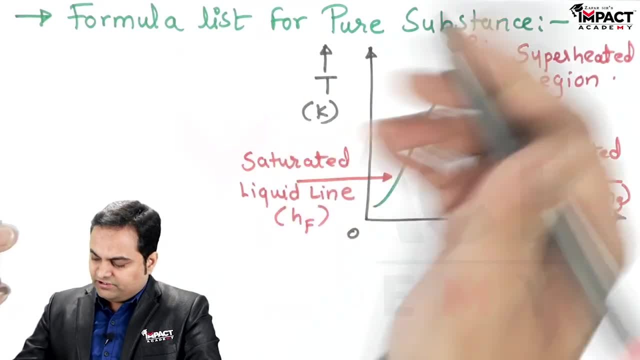 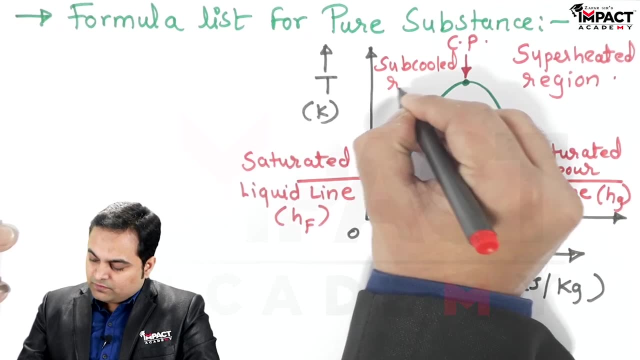 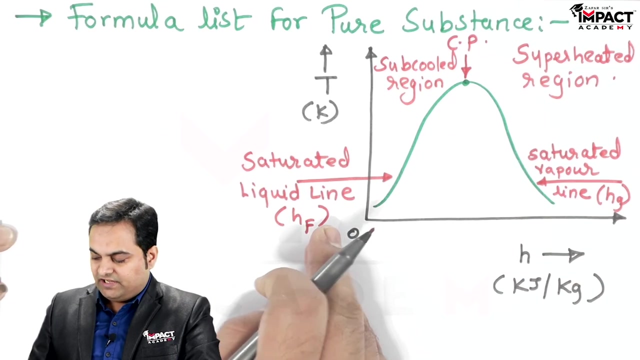 Similarly, just beyond this or before this saturated liquid line, The region which we have, it is called as the sub cooled region. Sub cooled region is below, we can say, the saturation point or the saturation liquid line, Like, for example, for water, since we know at atmospheric pressure it will boil at 100 degree Celsius. 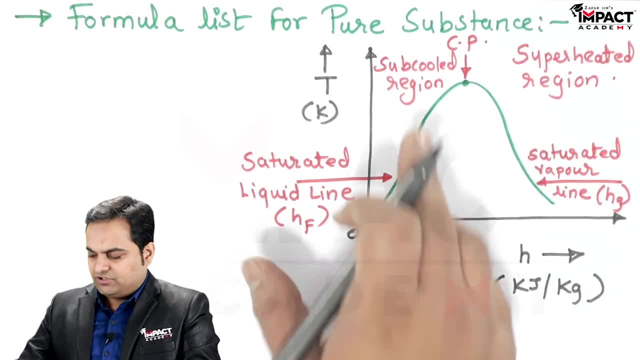 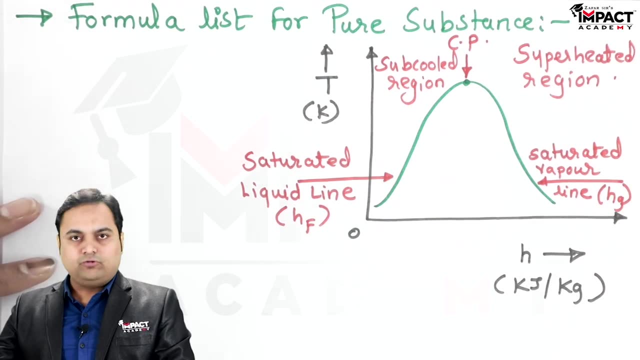 So any temperature below 100 degree Celsius at atmospheric pressure would go into the sub cooled region. Next, once we have understood these terms, And here the enthalpy of the superheated steam will be denoted by h- suffix superheated sup. 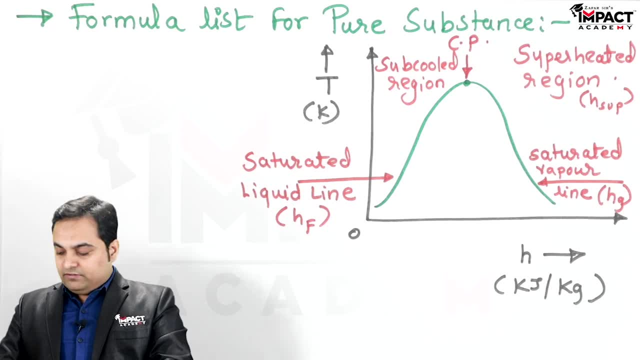 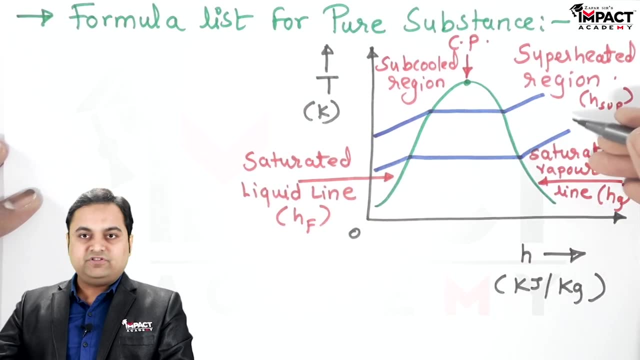 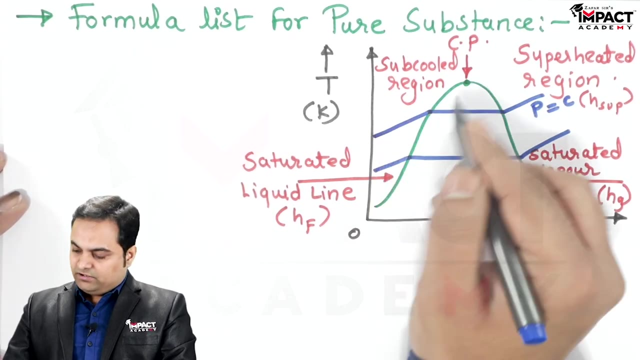 Enthalpy of superheated steam. Then I will be drawing the constant pressure lines over here, The lines which I am drawing. these are called as the constant pressure lines. So here, this is the higher pressure line. Now, when I take a point anywhere on this line, it will give me the same pressure value. 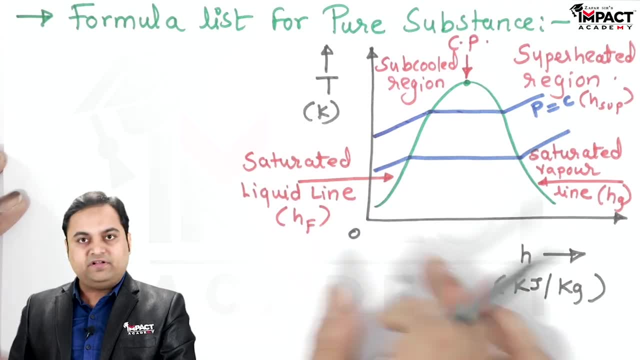 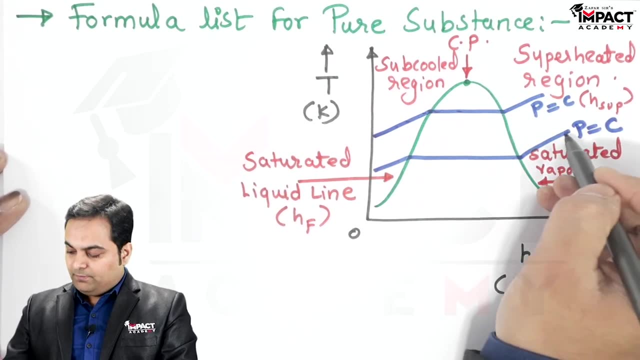 Because the pressure is not changing here And the enthalpy is changing. Pressure remains constant on this line, Similarly this bottom line. this is also having a constant pressure, But these pressure values are different for the lower region and for the higher region. 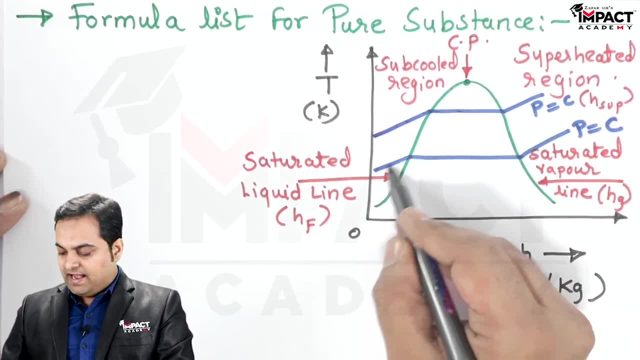 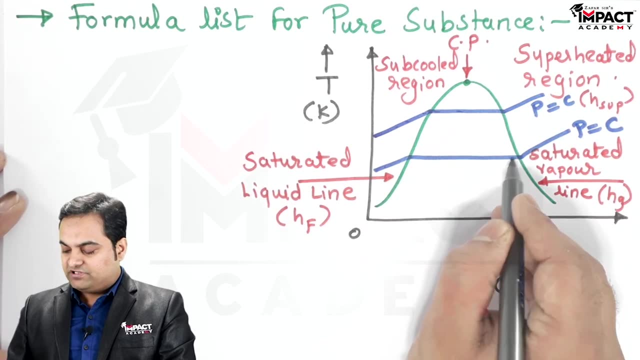 For example, the higher value of pressure can be boiler pressure And lower value of pressure can be condenser pressure. So these are two different pressures, But when you take any point on this line, on a particular pressure line, that will give you the same pressure. 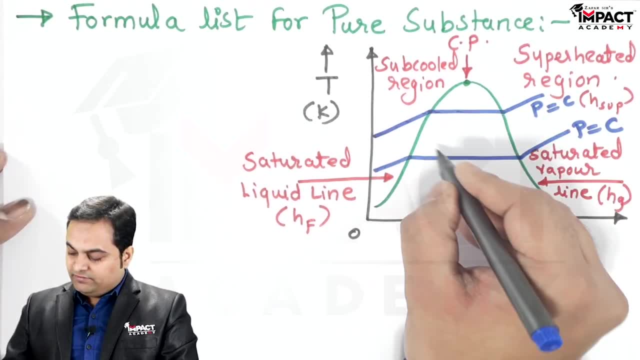 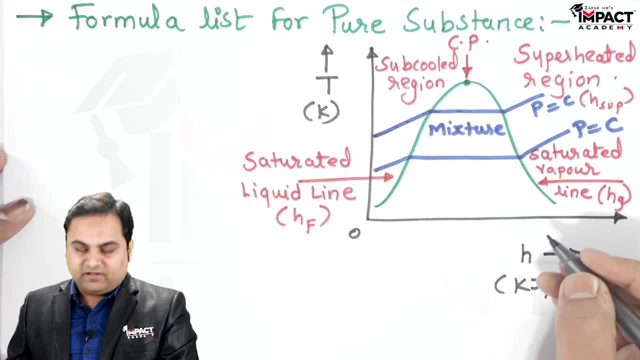 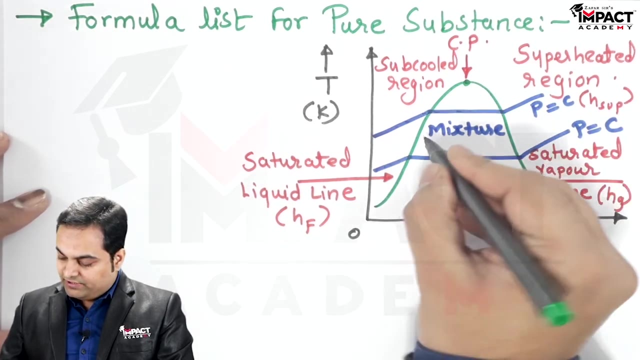 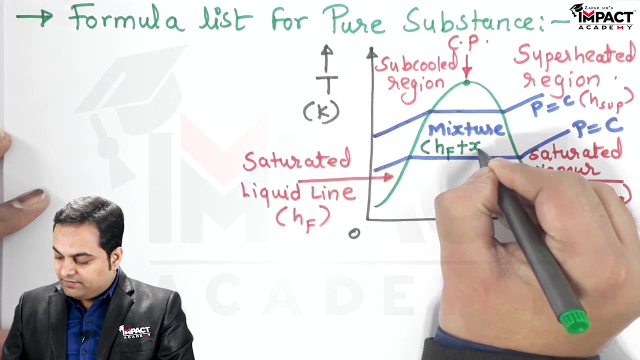 So that we have to remember The region which we have in between. that is called as the mixture region, And by mixture we mean that it is a mixture of water vapor plus dry air, So the enthalpy of water vapor. we know that it is denoted by hf plus. we have another term which is called as x into hfg. 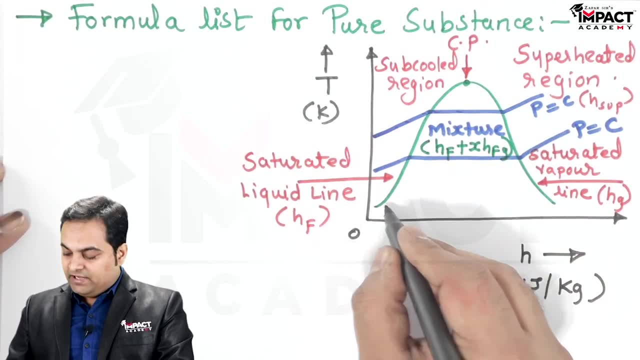 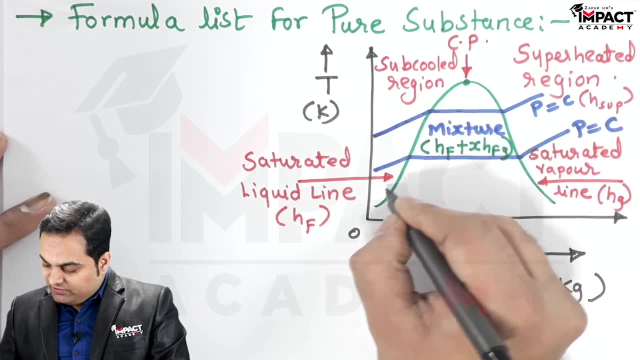 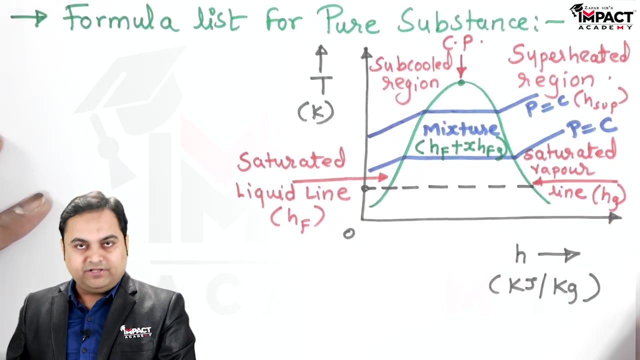 Where hfg is the amount of latent heat. And what is latent heat is that keeping the temperature constant. I am explaining on this graph that when we are keeping the temperature constant, Like indicated by this dotted line, The constant temperature by the horizontal line. 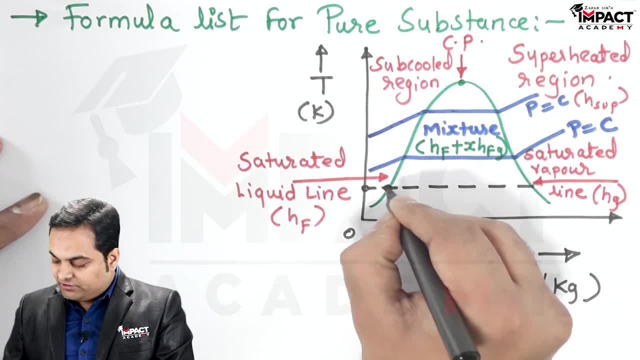 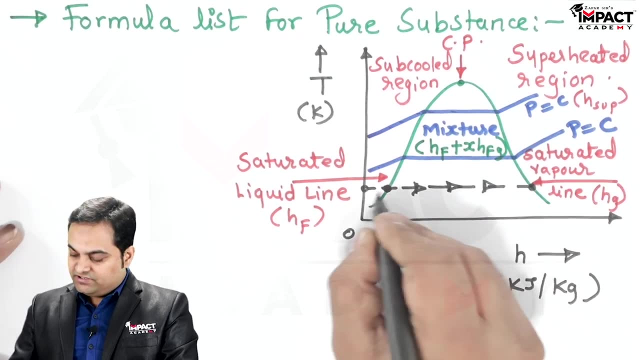 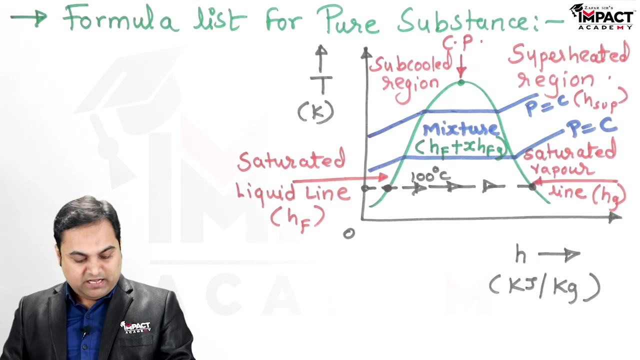 So we are crossing from the saturated liquid region towards the saturated vapor region, But there is no change in temperature. This is similar to the boiling of water at 100 degree Celsius. So the heat which is added, like, for example- I will show it over here on this graph. 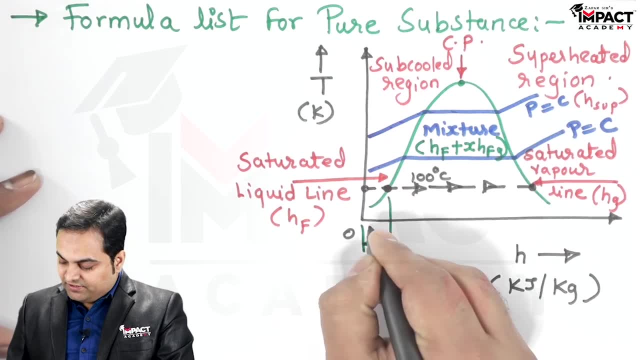 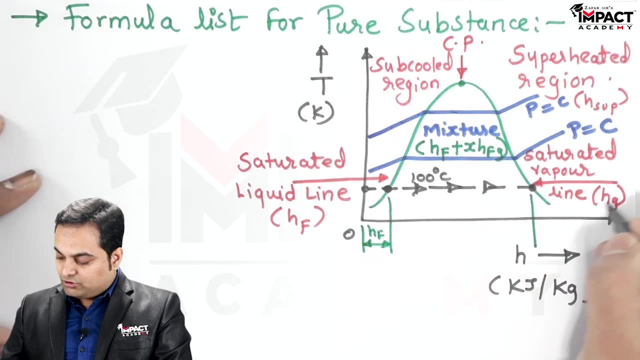 That initially the water which is at 100 degree Celsius. it has an enthalpy of hf. h suffix f over here. Now we have to add another enthalpy to this to get the answer of hg up till here. that is the final enthalpy. 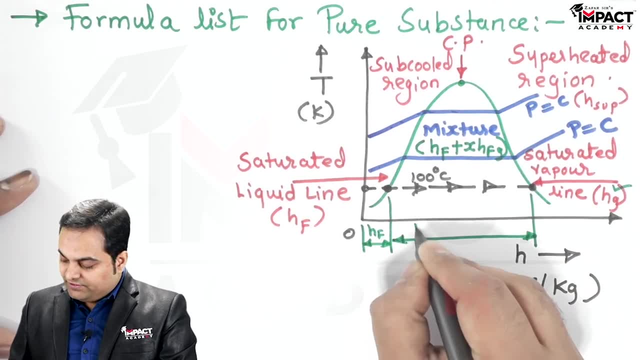 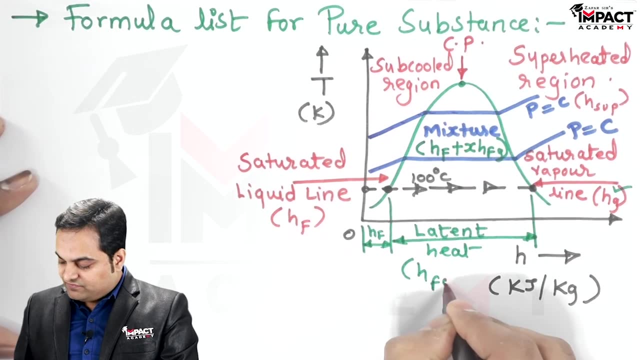 So we have to add this much amount of heat over here And this heat is called as the latent heat, which is in the mixture region. Latent heat is denoted by h suffix fg, that is hfg, the enthalpy of latent heat. 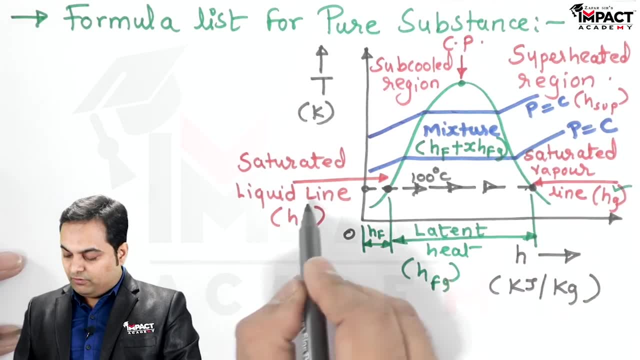 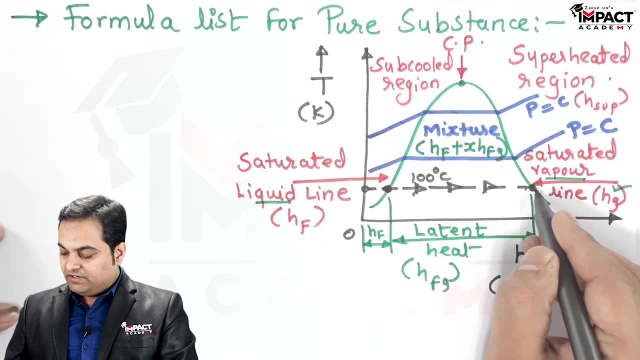 So latent heat is that heat which causes the change of phase from liquid to vapor without changing the temperature. So that is the latent heat and it goes into the dry region that is hg. So I will explain the formula one by one once we have understood this graph. 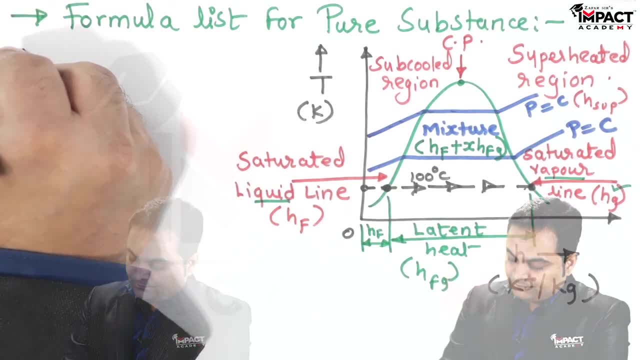 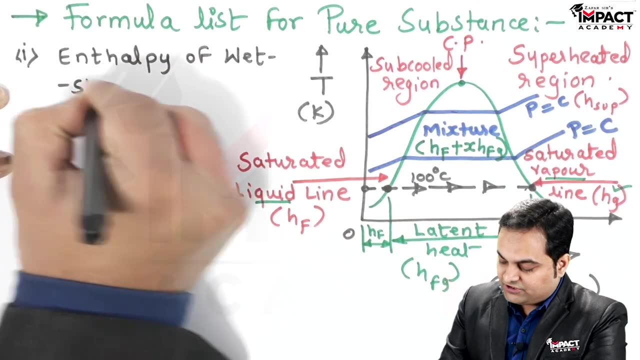 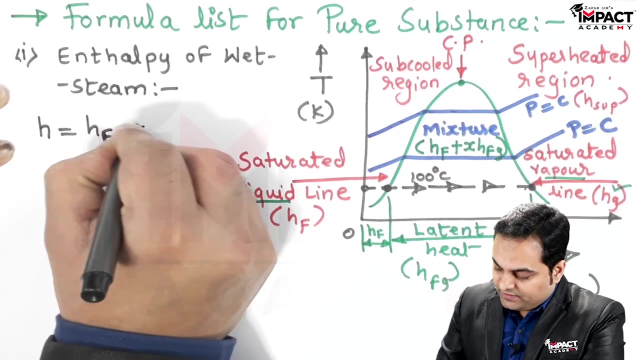 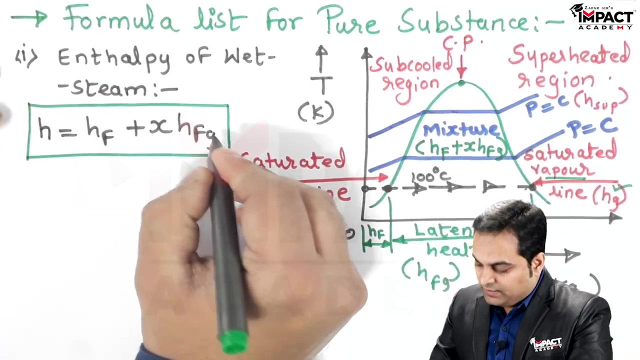 Starting with the first formula, The enthalpy of wet steam. So wet steam enthalpy denoted by small h, given by the formula, it is hf plus x into hfg And the unit would be in terms of kilo joule per kg specific enthalpy. that is why the notation is small h. 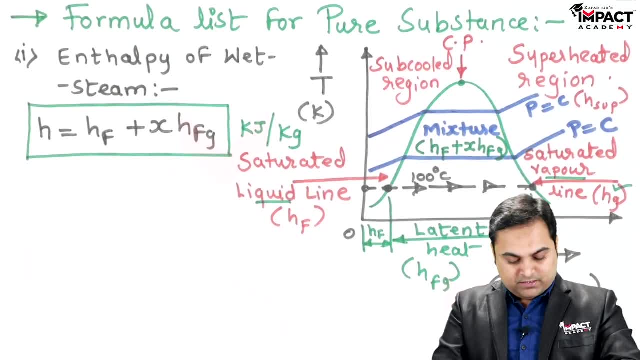 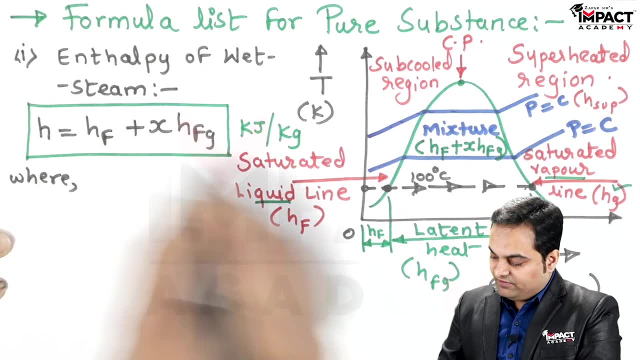 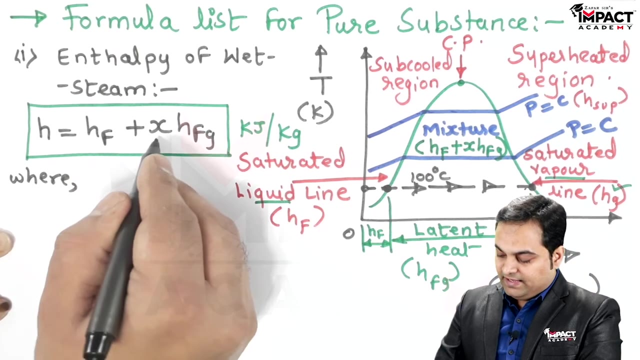 If it is total enthalpy, the unit would have been capital H. So here I can say that where hf is the enthalpy of saturated liquid Hg, hfg is the latent enthalpy and x is the dryness fraction. 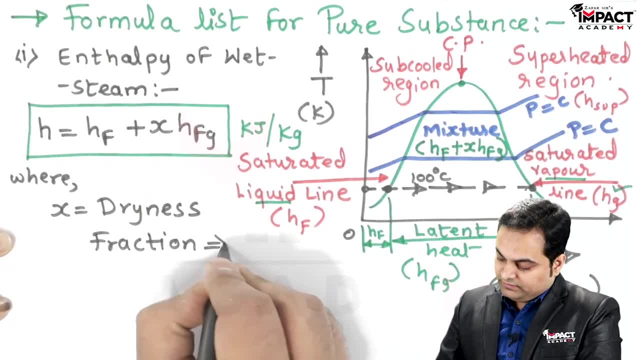 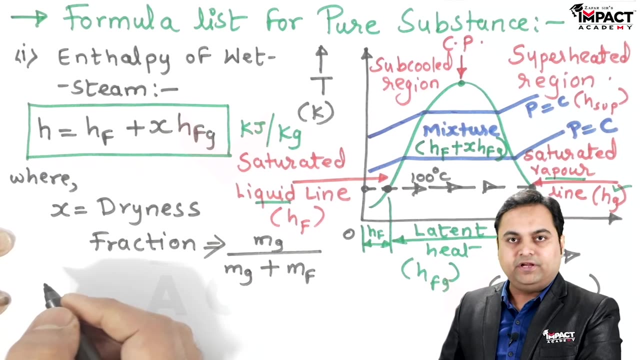 Dryness fraction is given by the mass of dry air upon the mass of dry air, plus mf, the mass of water vapor in the air, Because air contains both dry air as well as water vapor. So we have to add both the masses and the mass of dry air upon the mass of total mass of air. that gives us the dryness fraction. 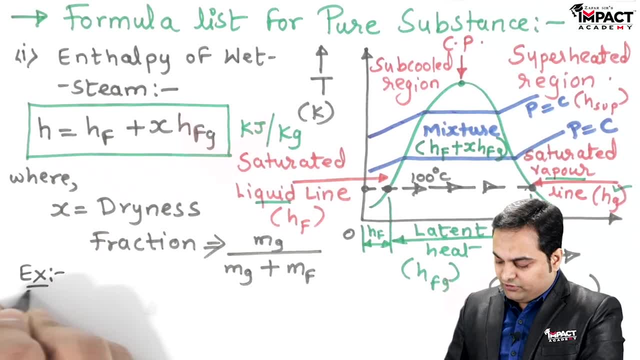 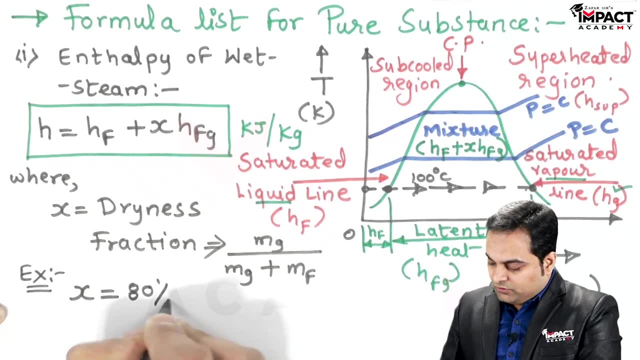 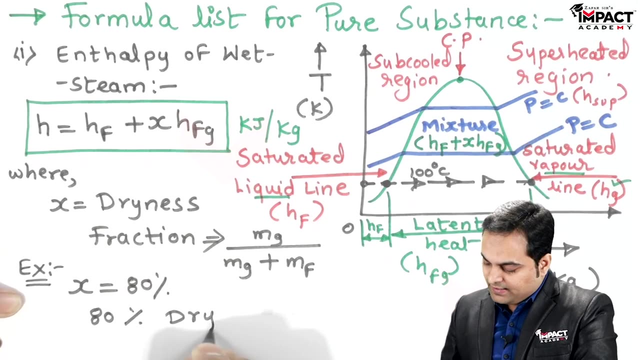 And what is this dryness fraction? I will explain with an example. Like, for example, for any given steam, The dryness fraction is given as 80%, So that 80% means the steam is 80% dry and it contains 20% water vapor. 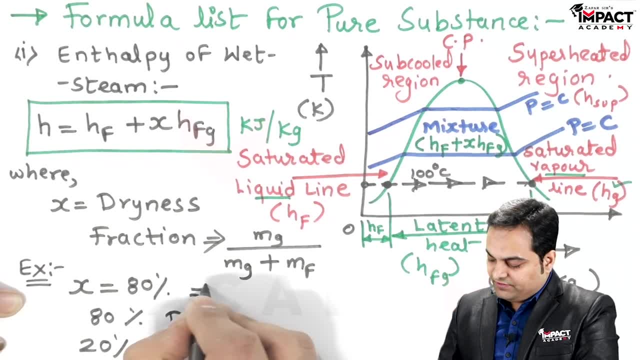 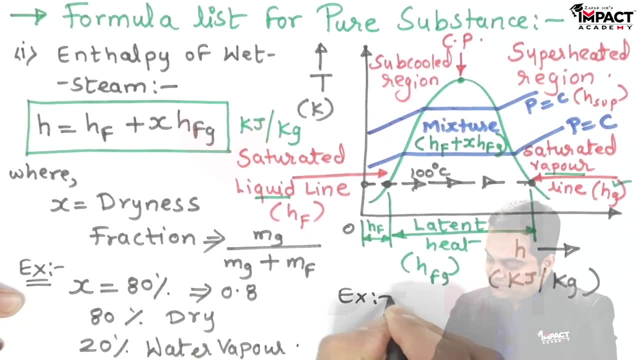 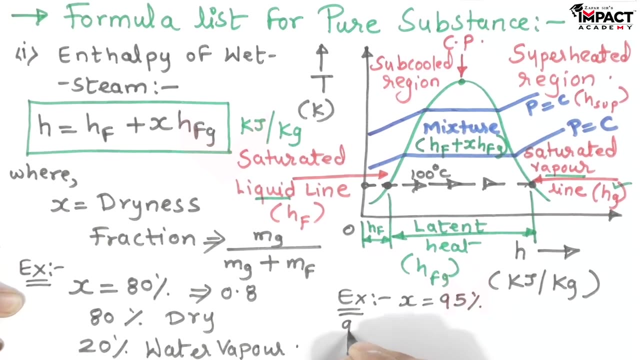 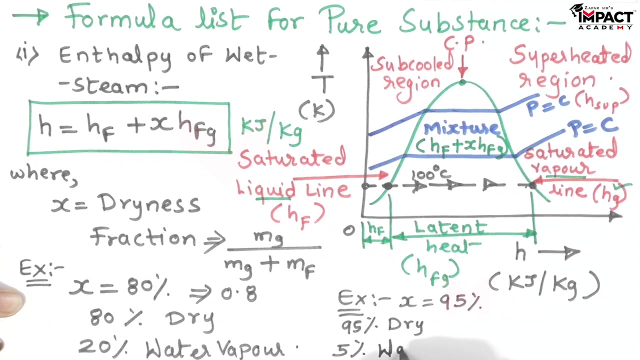 And this dryness fraction, when written in the form of number, it would be 0.8.. Similarly, if, for example, the dryness fraction is x equal to 95%, So it means it is having vapor which is 95% dry and 5% wet, or we can say 5% water vapor. 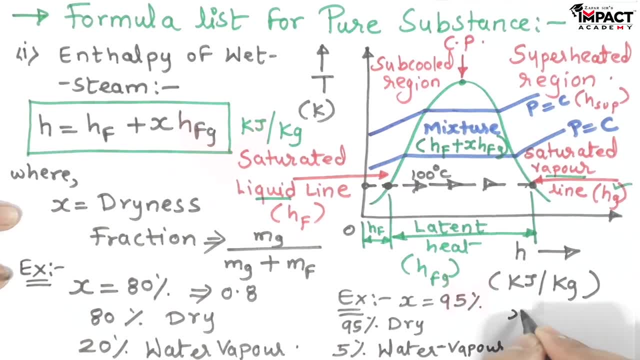 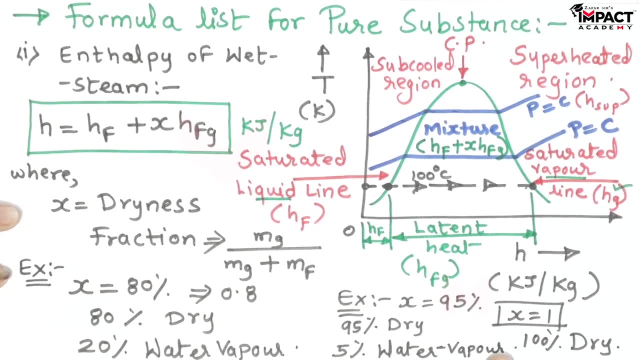 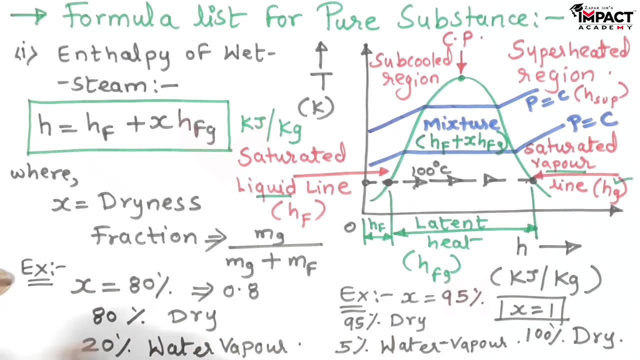 And if the dryness fraction x is equal to 1. It means that steam is 100% dry And that is no water vapor is present in that steam. So dryness fraction, as we see here, if the value, we can simply say, if the value of dryness fraction is less than 1.. 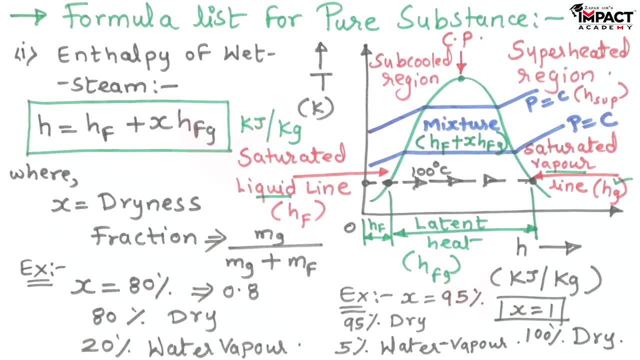 It means the steam is wet steam, as simple as that. And if the dryness fraction is equal to 1, it means it is dry steam. So in the same formula, when I put x equal to 1. I will be getting the enthalpy of dry steam which I am going to write now. 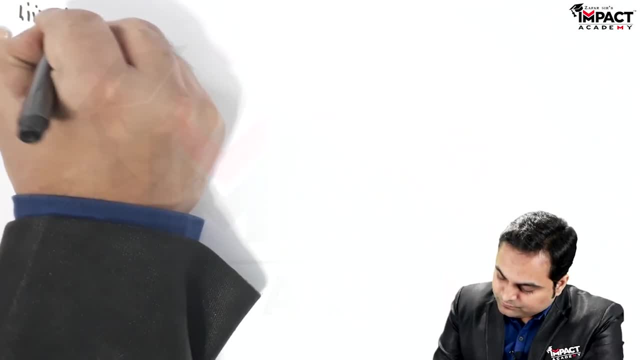 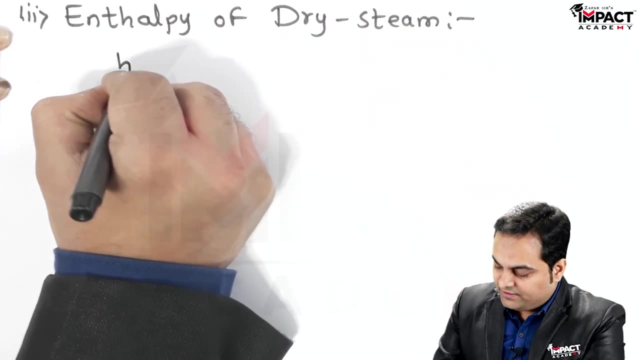 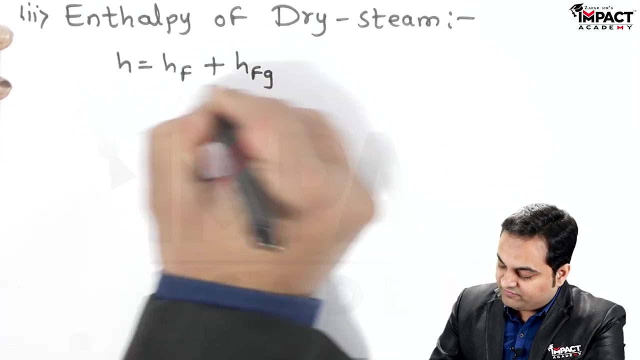 So this is the enthalpy of wet steam. Next Enthalpy of dry steam, which is 100% dry, is given by: h, is equal to hf plus now x value would be 1.. So it is hf plus hfg because x value is 1 and that is for dry steam. 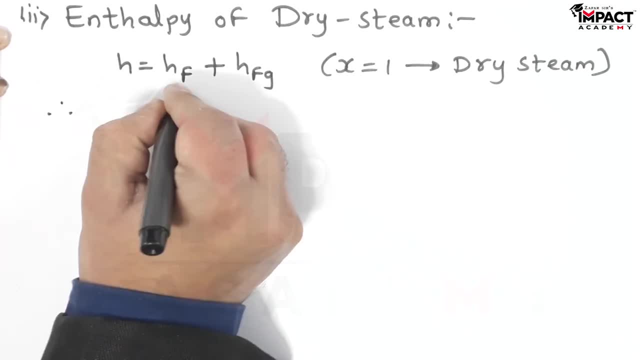 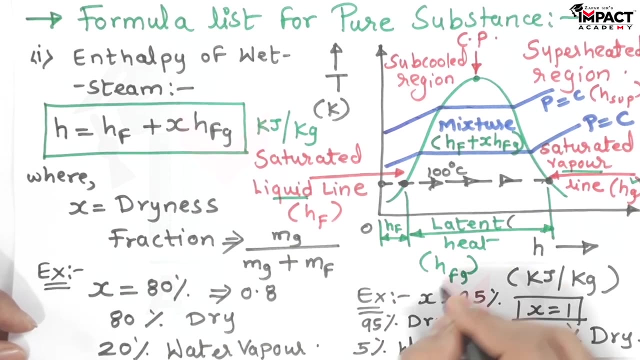 The dryness fraction is 1 and therefore when hf and hfg gets added- So here we can see from the graph- hf plus latent heat is denoted by hfg. So hf plus hfg, when gets added, they give us the value of hg. 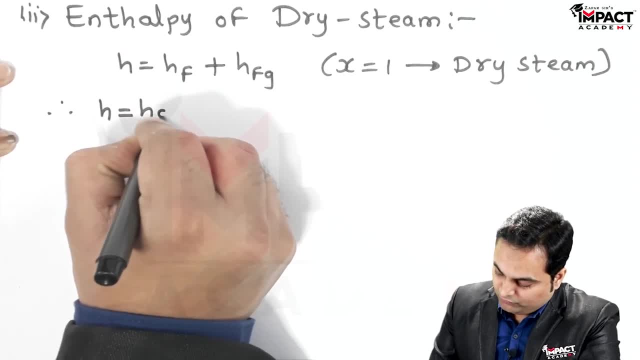 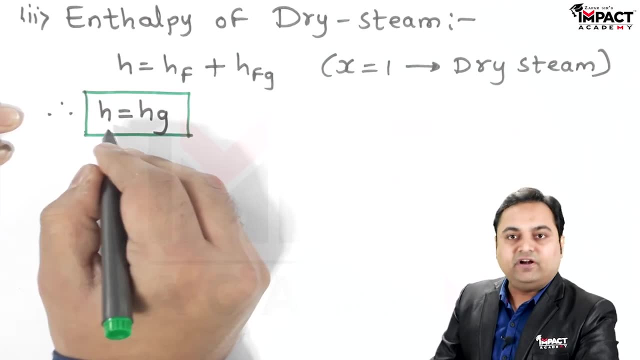 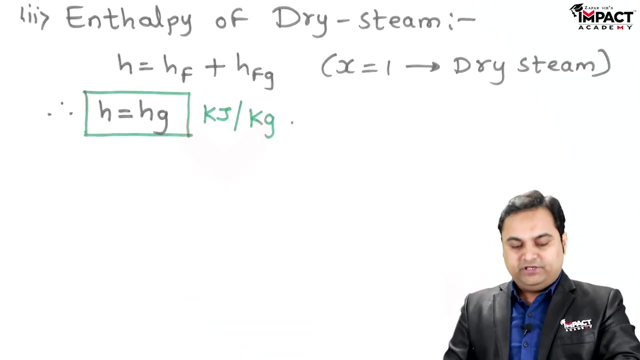 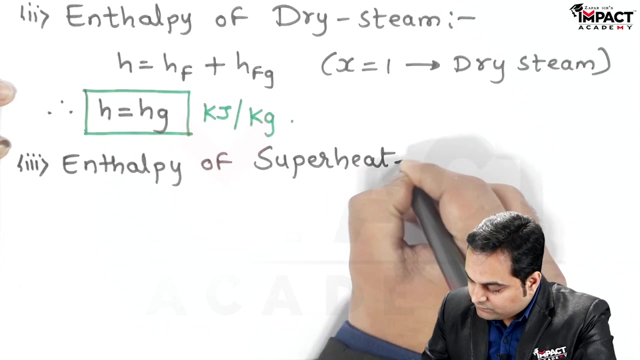 So therefore, the enthalpy of dry steam would be denoted by h suffix g, And this we can find it from the steam table Unit is kilo joule per gauge. Next, the enthalpy of superheated steam. Superheated steam, we know the temperature of the steam will be above 100 degree Celsius. 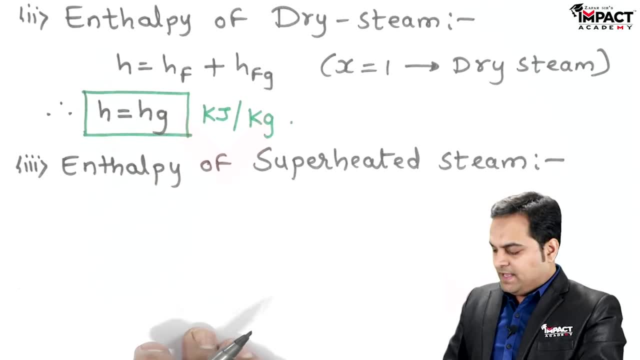 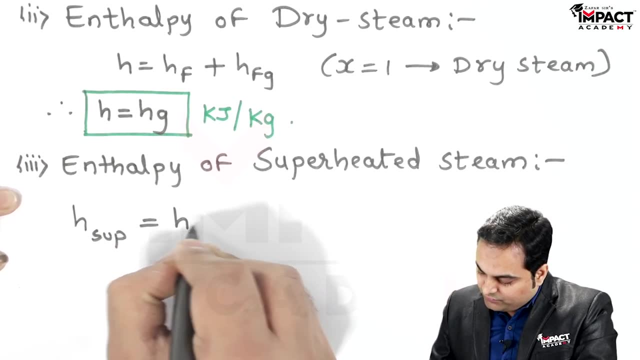 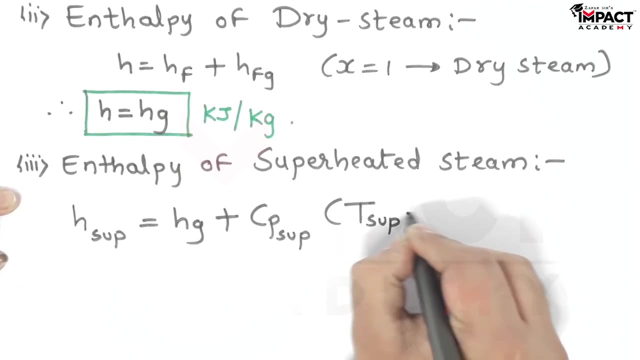 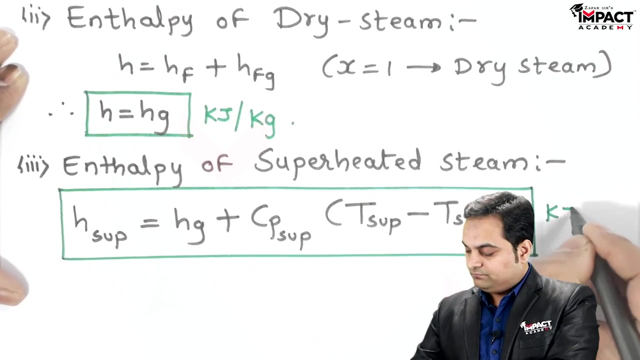 That is above the saturation temperature of water at atmospheric pressure And that enthalpy is given by the notation is h suffix sup And that is equal to hg plus specific heat superheated into T superheated minus T saturated, It means when we go into the superheated region. 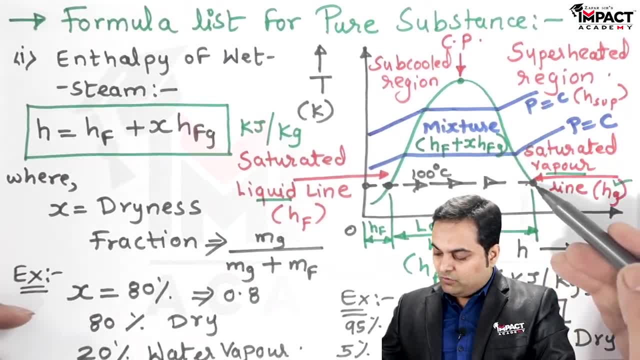 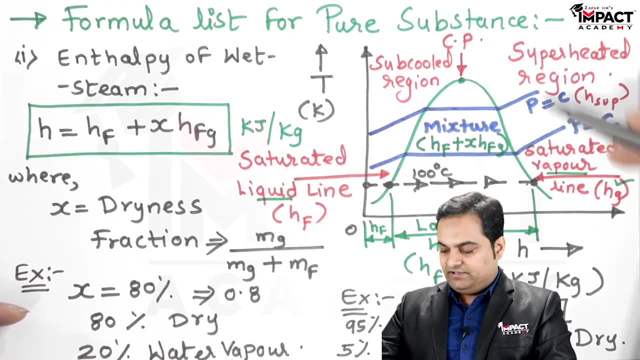 Then we have to at least reach first the saturated vapor line, that is hg value, And beyond that we have to add the degree of superheat. So that is the enthalpy of the superheated steam And hg, we know it is the enthalpy of the dry steam. 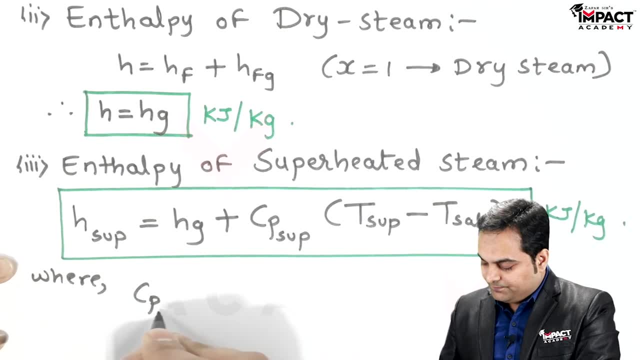 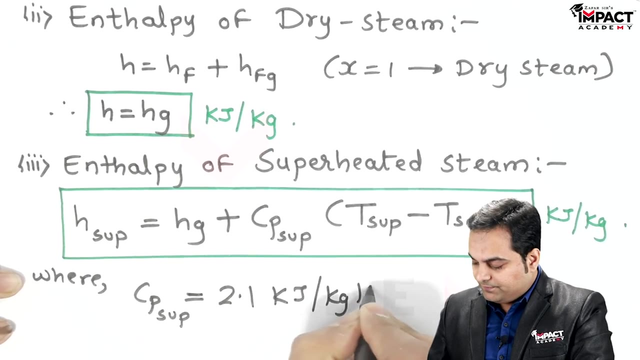 Where specific heat, Cp superheated- Is the specific heat of that steam at constant pressure And this value is constant. for steam You can take the value as 2.1 kilo joule per kg kelvin. So this value you can just remember for steam. 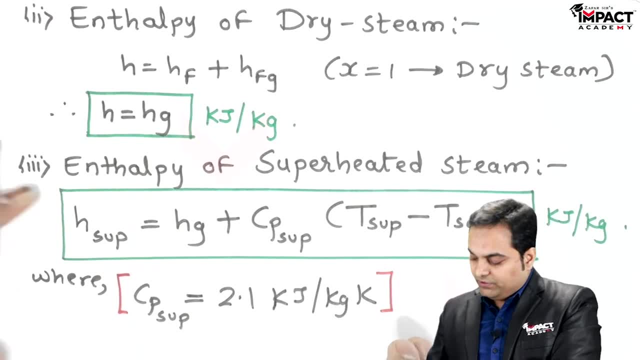 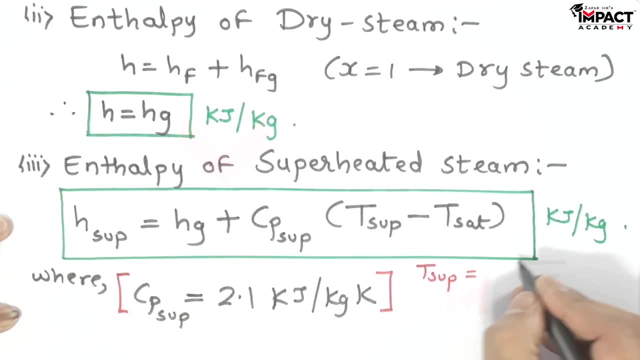 The specific heat of superheated steam is given by 2.1 kilo joule per kg kelvin. Next T, superheated, It is the superheated temperature, The temperature of the steam, And since here we have temperature difference, 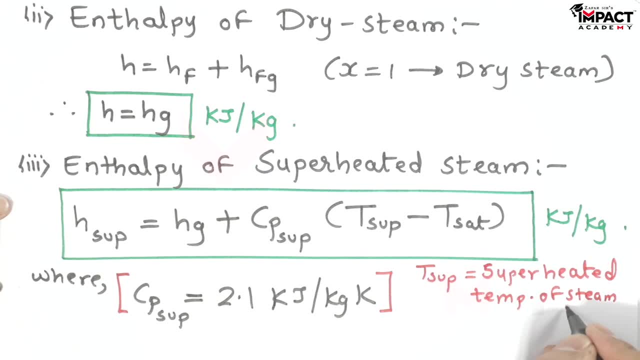 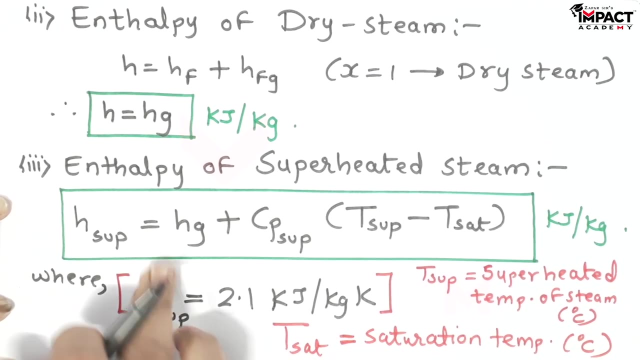 It doesn't matter when we keep the temperature in terms of degree Celsius or kelvin, I am writing it in terms of degree Celsius. Similarly, T saturated: It is the saturation temperature of steam And that is also in terms of degree Celsius. So first we have to have dry steam. 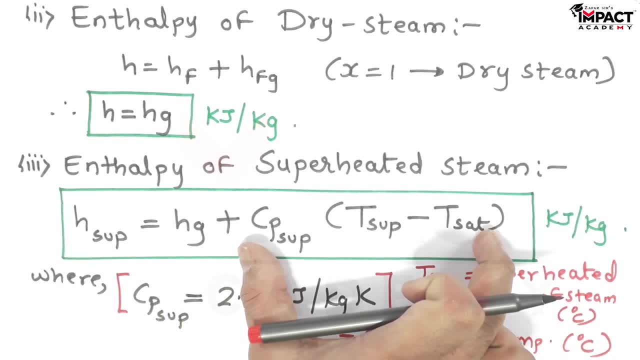 Then we have to add this much amount of heat, That is, specific heat superheated, into this difference And then it will become the superheated steam. So enthalpy of superheated steam can be calculated in this way, And this bracket: T superheated, minus T saturated. 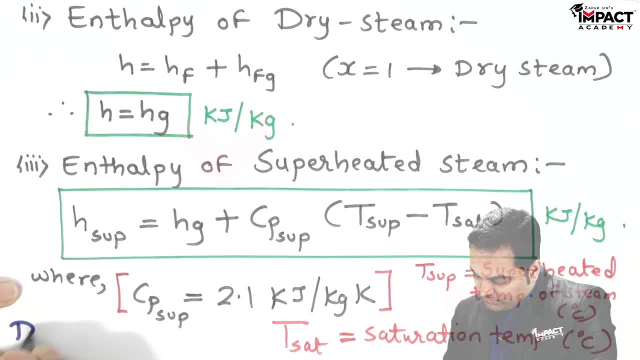 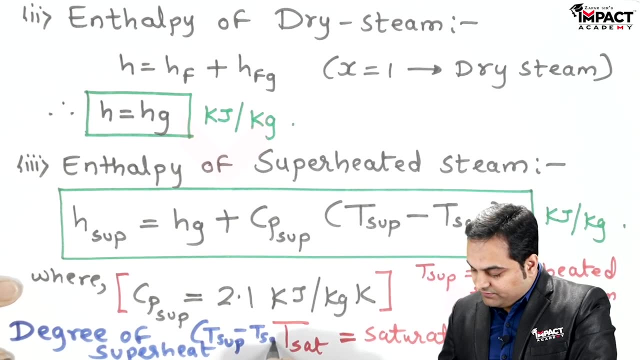 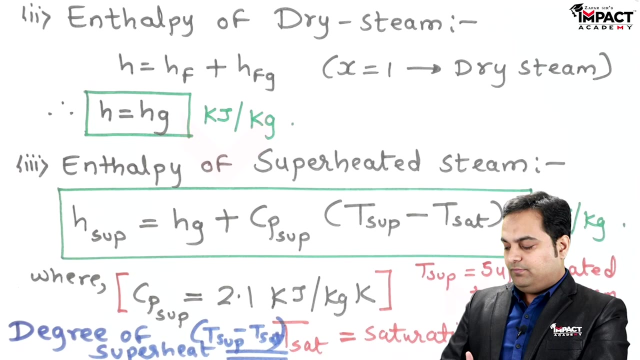 That is called as degree of superheat: T superheated minus T saturated, That is the degree of superheat, So we can make out how much that steam is superheated. Next, after getting all the enthalpy, is here: 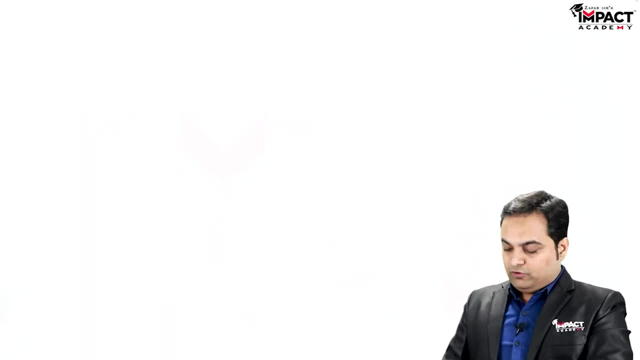 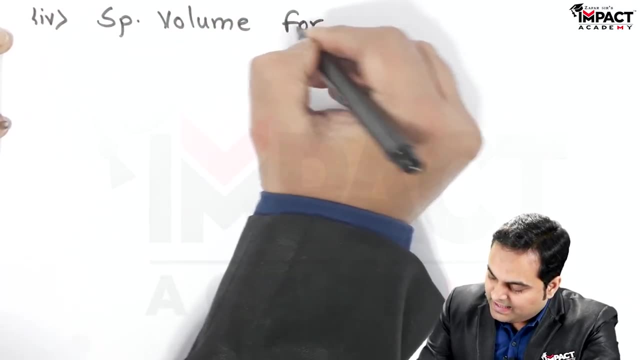 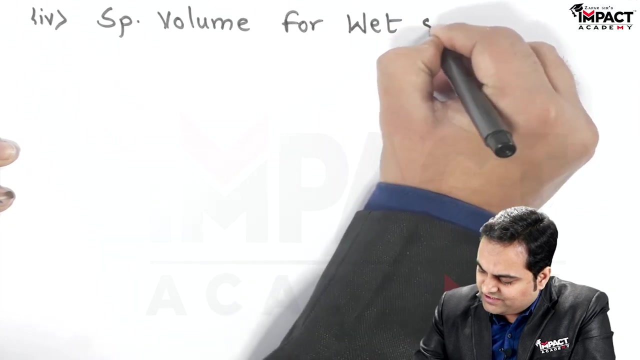 The next formula would be For specific volume of dry steam. And just before going for dry steam First, I will explain for wet steam, Specific volume for wet steam, So that we can understand dry steam more clearly. So how much would be the specific volume for wet steam? 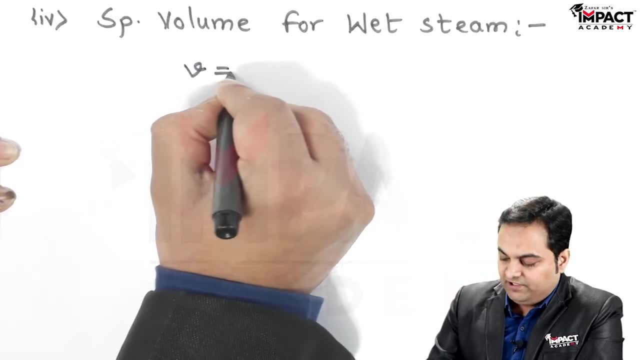 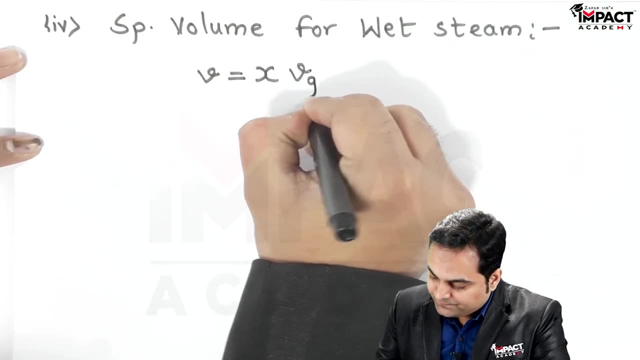 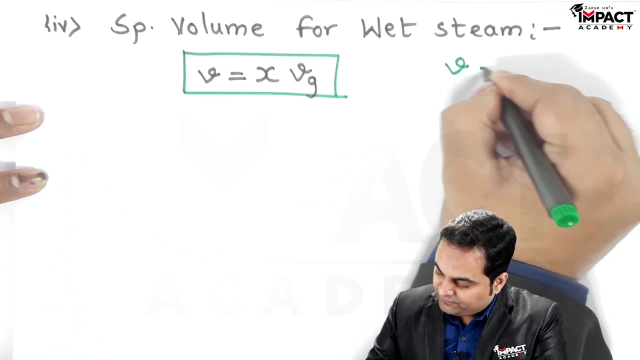 Specific volume is denoted by small v. So specific volume of wet steam, That is given by x into vg. Now, specific volume, It is the reciprocal of density. Specific volume is denoted by 1 upon rho. That is the reciprocal of density. 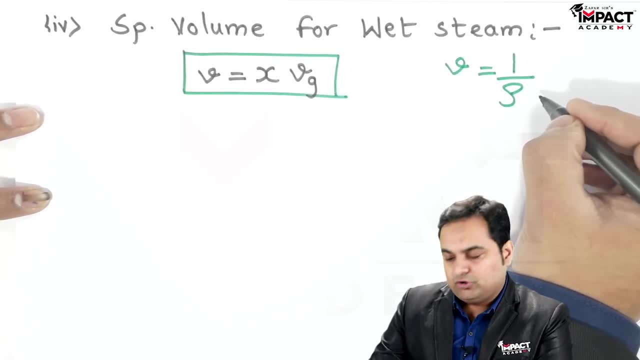 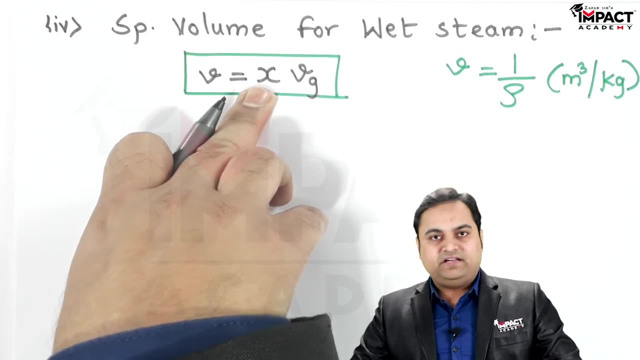 Density is having the unit of kg per meter cube. So when it becomes reciprocal, The unit is meter cube per kg And x, as we know it, is the dryness fraction. Vg is the specific volume of dry steam. Dry steam means: 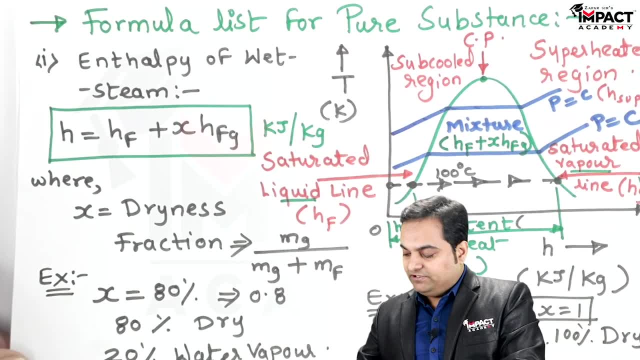 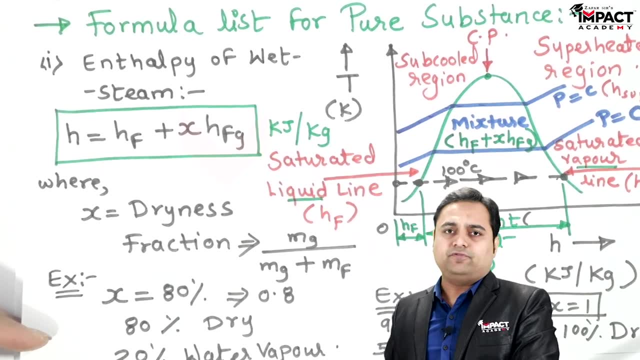 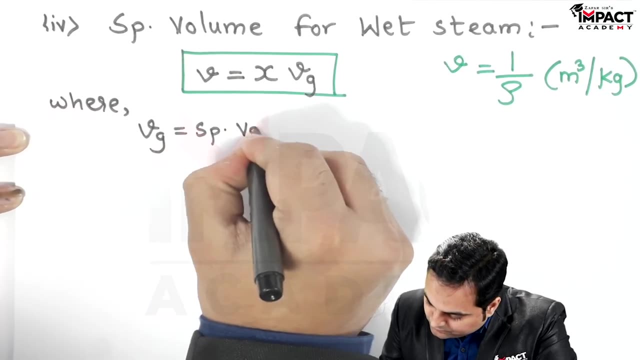 It is the dry saturated steam And we are going to get the value Like, for example, on this saturation curve. We are getting heg value, Similarly vg value. we can get it from the steam table. So that is the specific volume Of dry steam. 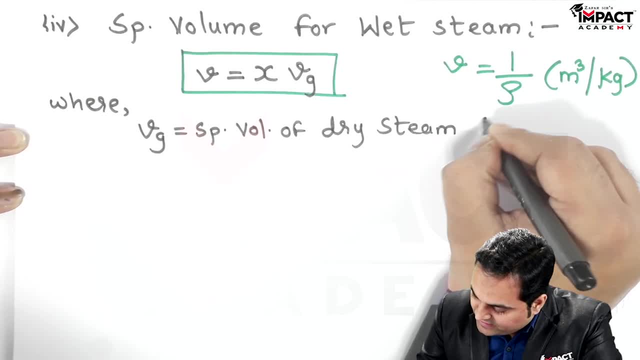 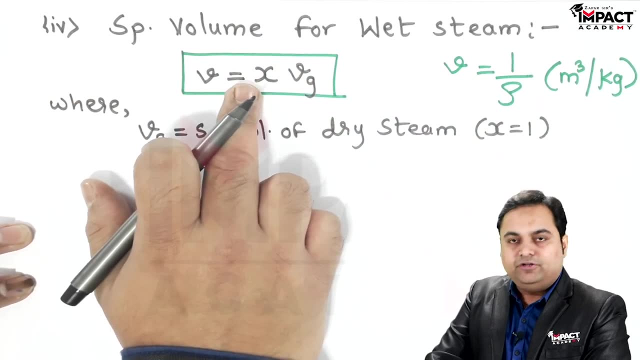 And for dry steam, we know that Dryness fraction will be equal to 1.. And for wet steam, When we want to calculate the specific volume x value, we know it will be less than 1.. So multiply the dryness fraction with vg. 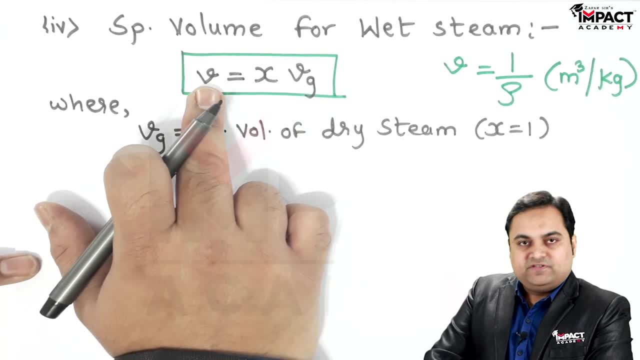 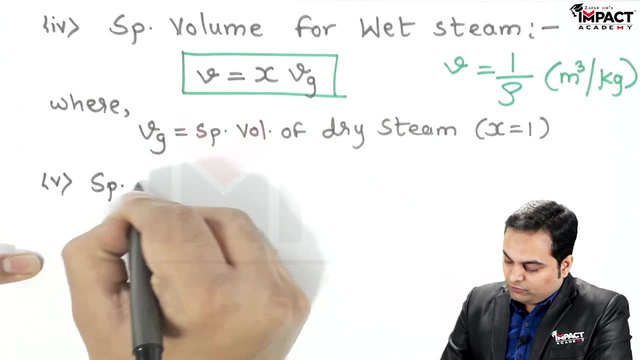 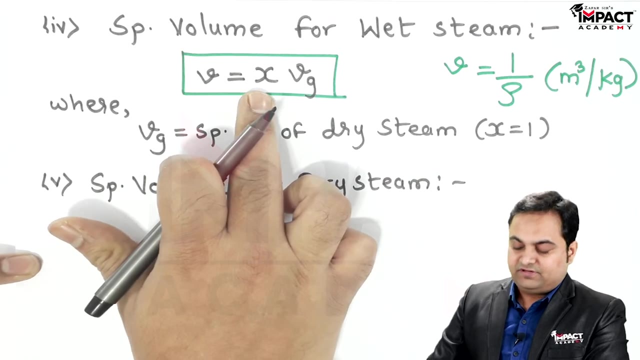 That is the specific volume of dry steam. We get the specific volume of wet steam. Now, after that Specific volume For dry steam, We will get the dry steam. Simply put The dryness fraction as 1. So when x is equal to 1.. 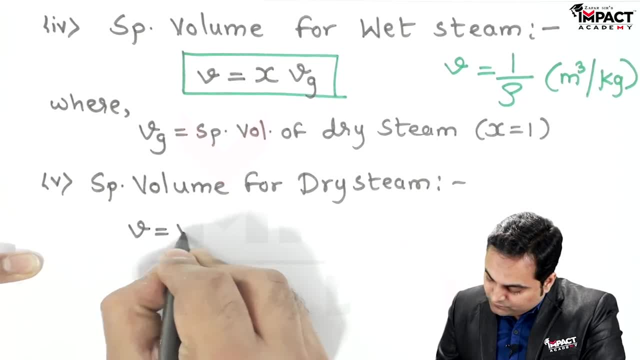 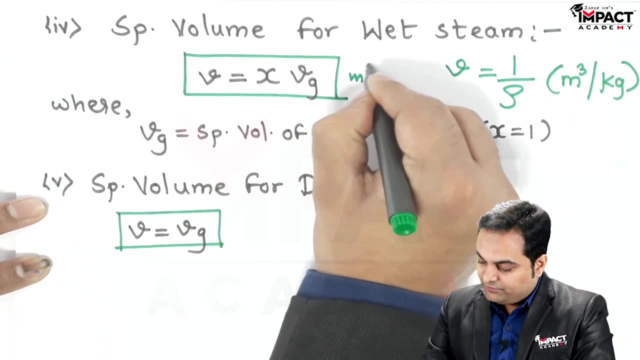 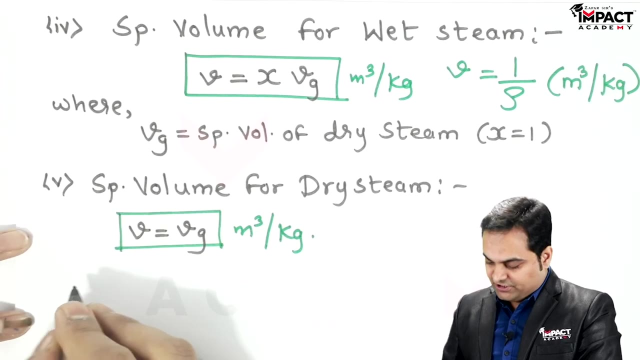 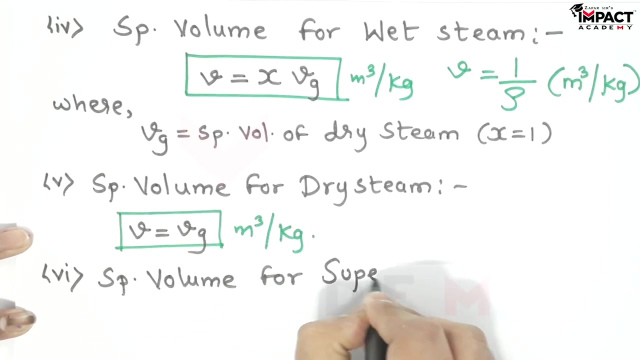 Specific volume is equal to vg. That is the specific volume of the dry steam Unit in terms of meter cube per kg. Now next is The specific volume of superheated steam Which is heated above the saturation temperature. It can be found from a simple relation. 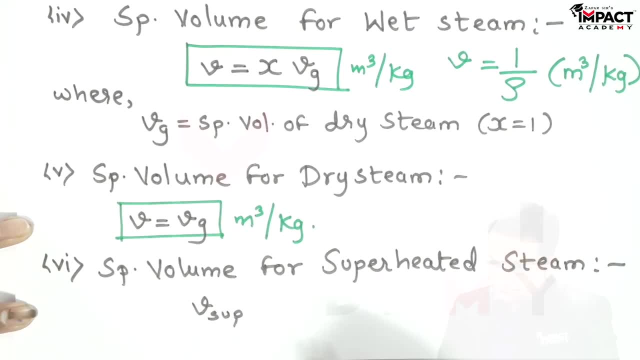 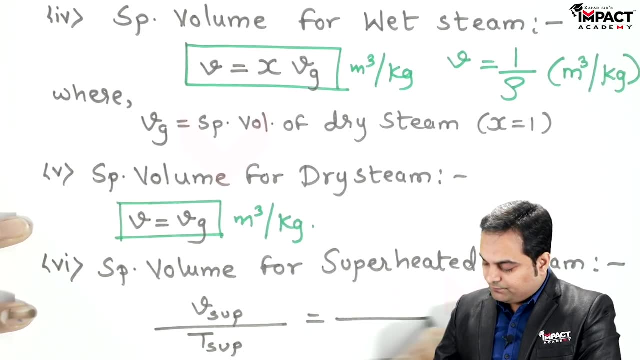 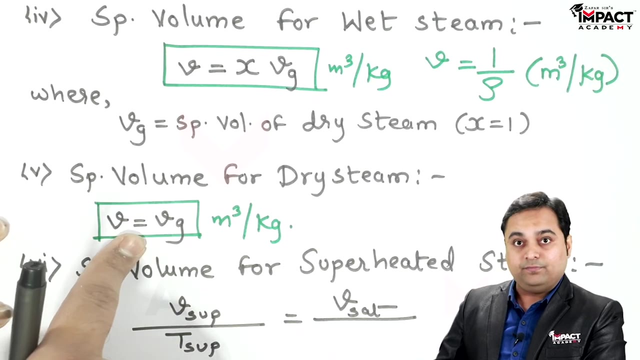 Like specific volume of superheated Upon the temperature of The superheated steam, Is equal to The specific volume of Saturated steam, Which can be the dry steam Having vg value Upon the temperature of saturation Saturated steam. 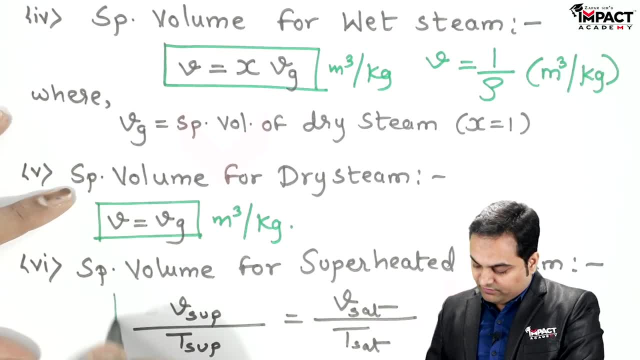 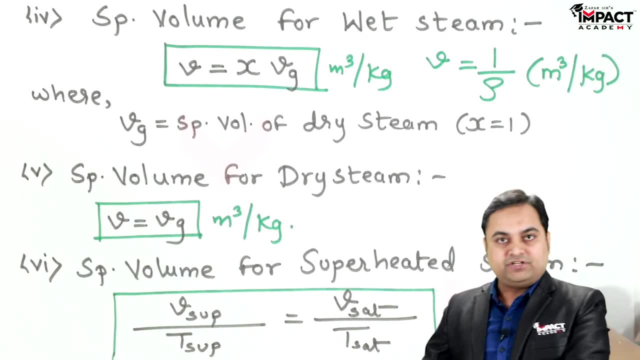 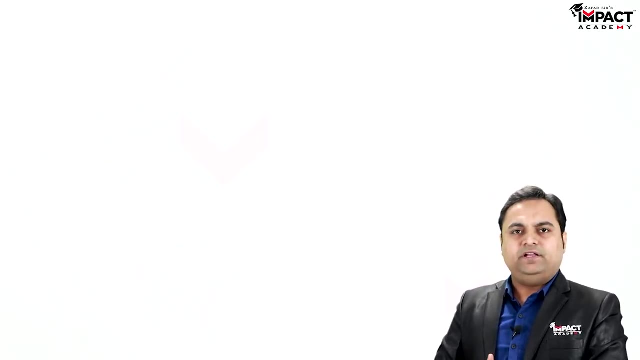 So also we can say the dry steam. By using this simple concept of Like, we can say similarity. We can find the specific volume of The superheated steam. Next, In a similar manner, I will be explaining the entropy formula. 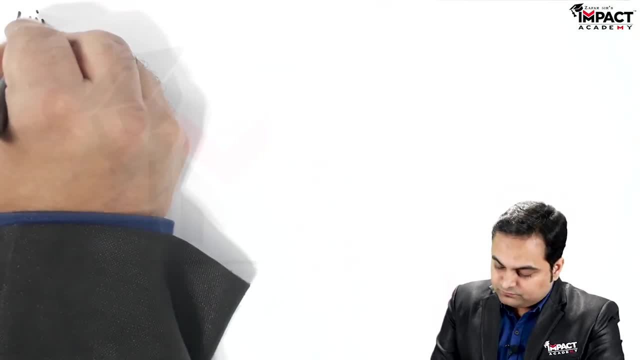 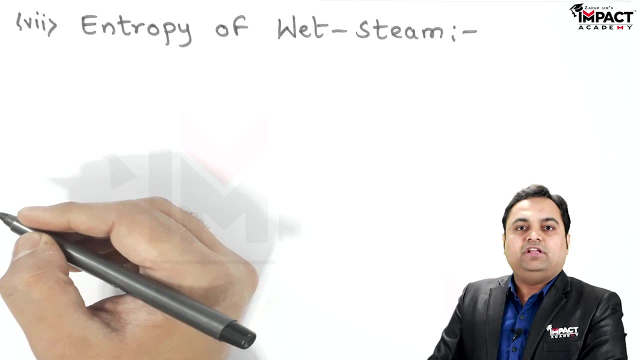 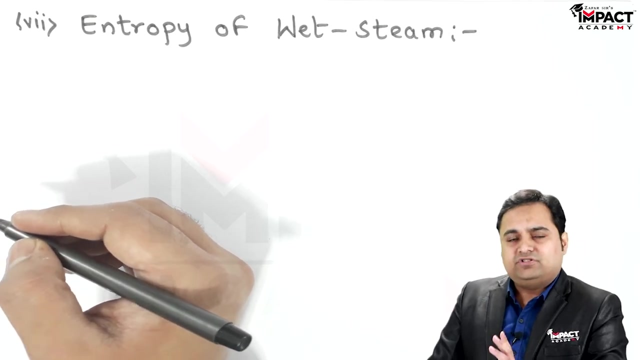 Like I had explained, the enthalpy, Now The entropy of wet steam, And remember these are The specific properties, Means the unit would be always In the form of per kg, Because the steam table is made on per kg basis. 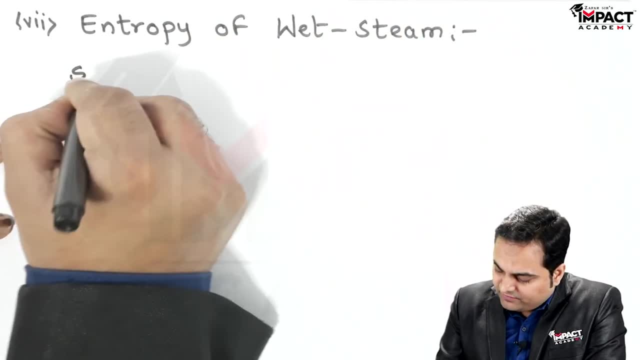 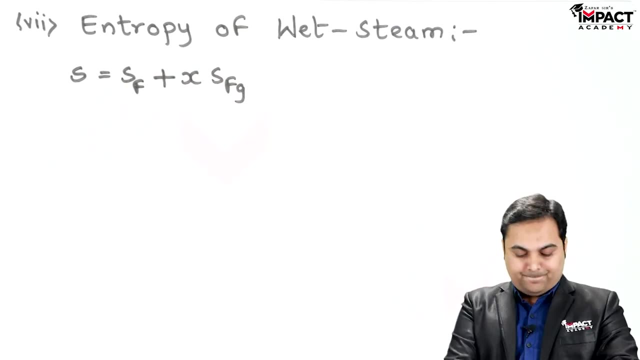 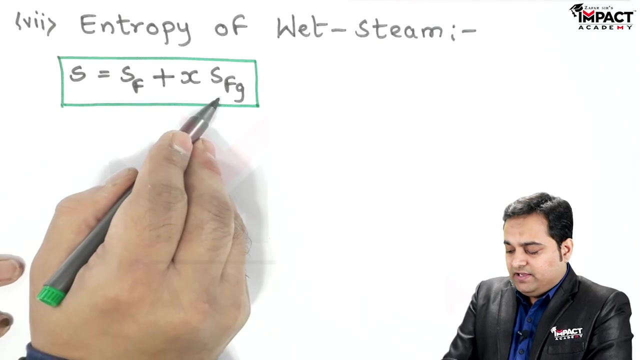 So specific entropy of wet steam Denoted by s suffix, It is s and written as Sf plus x Into sfg, Where sf is The entropy of the liquid Which is saturated liquid, Sfg is the latent entropy. 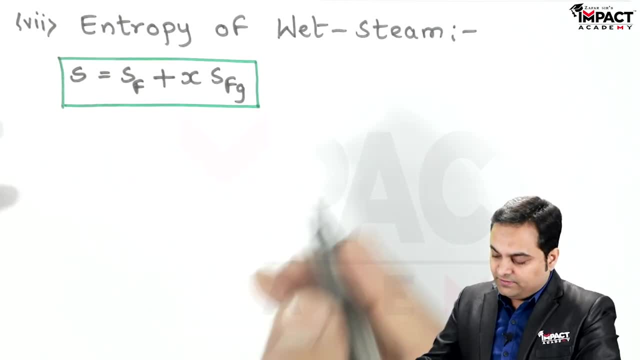 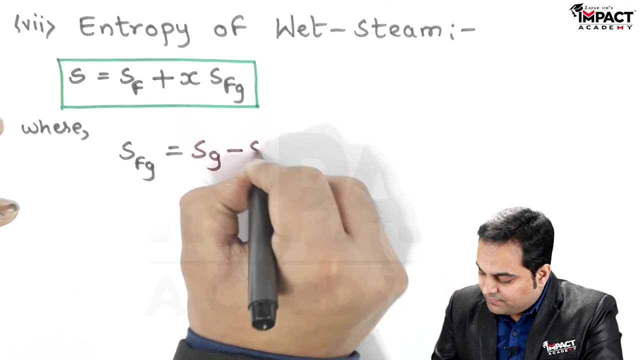 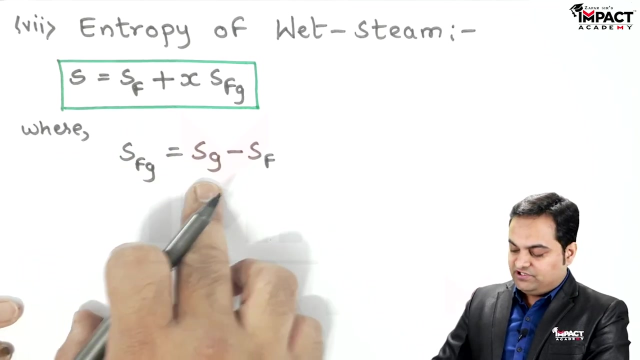 And here we can also say that Sfg Can also be Set as Sg minus sf, Because basically Sg is Sf plus sfg, So sfg is sg minus sf. So sometimes we may use: 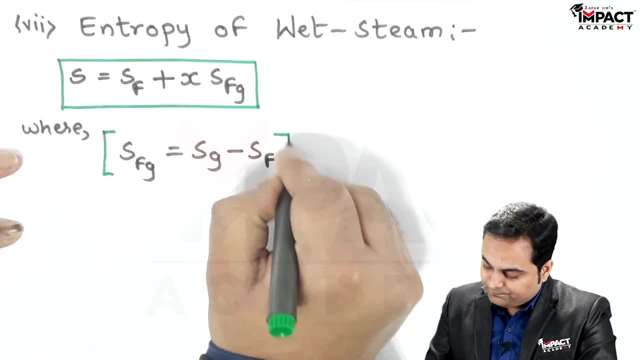 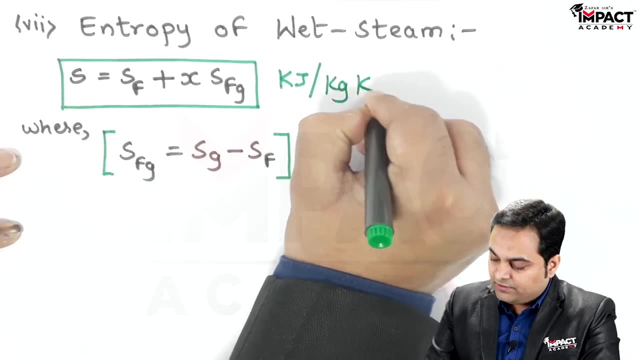 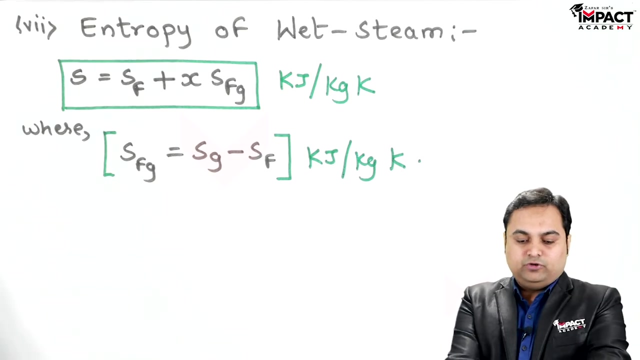 This relation as well, While solving the problem. And the unit is, As I have said, Per kg, basis specific unit, So kJ per kg kelvin. Similarly, here also it is kJ per kg kelvin. And previously, Where I had explained enthalpy also. 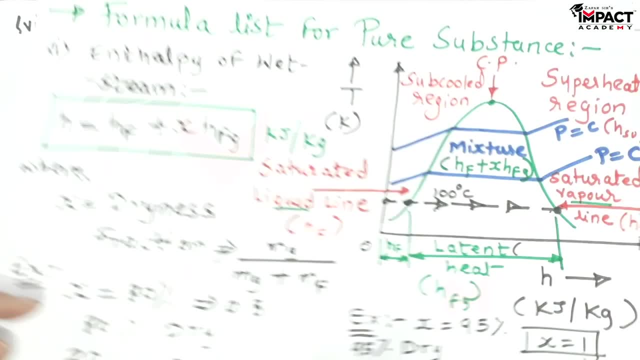 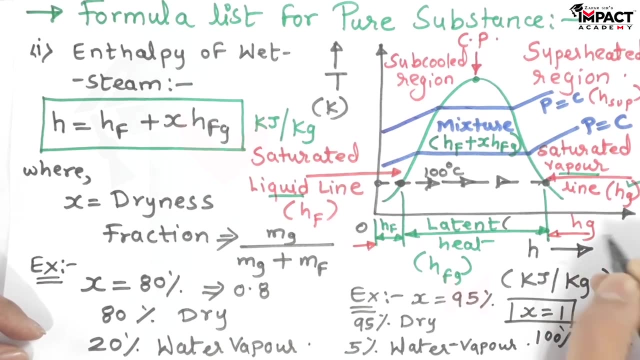 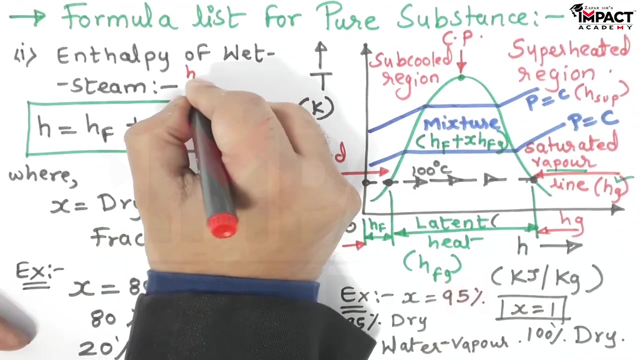 I will write there as well That Sfg can be Set as hg, Because hg is the total value Which is made up of Sf plus sfg. So Sfg Will be equal to Hg minus hf. 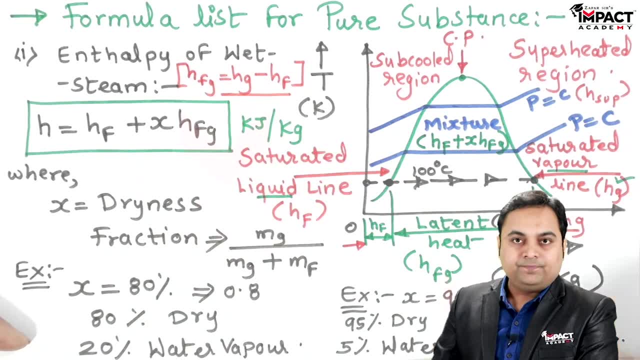 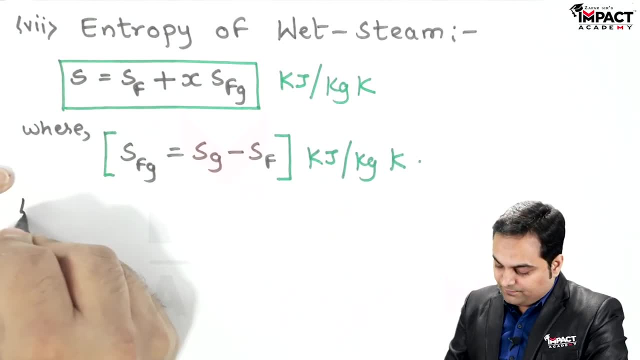 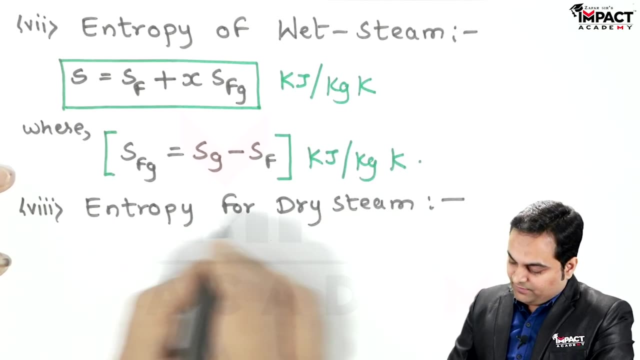 The latent Enthalpy over here. Now, After getting this, The specific entropy of wet steam. Similarly for dry steam. For dry steam It would be denoted by s Suffix g. And how this comes I will explain. 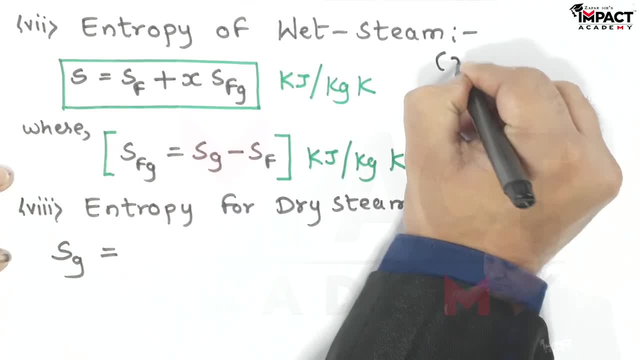 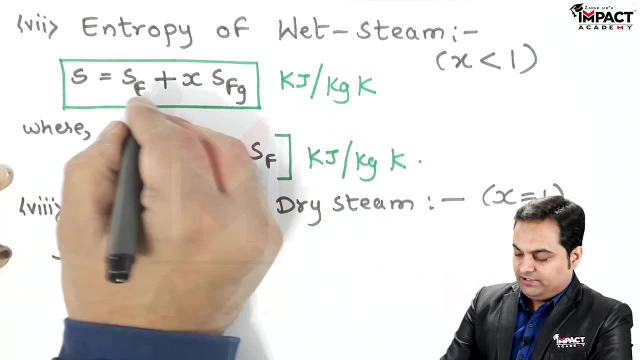 That Dryness fraction is equal to 1. And if it is wet The dryness fraction is Less than 1.. So when I keep the value as 1., It is sf plus sfg And we know that.